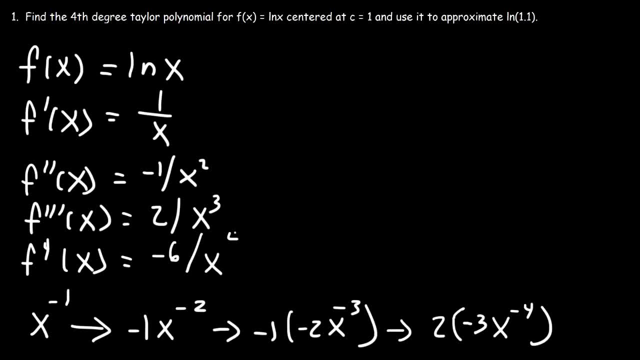 So this becomes negative 6 divided by x to the fourth power. Now f of 1 or f of c, because c is 1.. That's the natural log of 1, which is 0. And then f, prime of 1.. 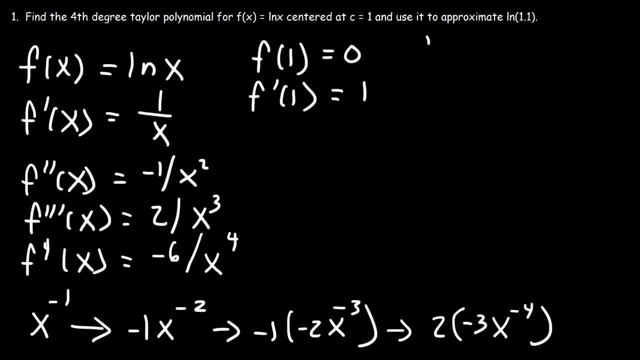 That's going to be 1 over 1, so that's simply 1.. And then f, double prime of 1. If we plug it into negative 1 over x squared, that's just going to be negative 1.. And then for the third derivative, that's 2 over 1 cubed, so that's simply 2.. 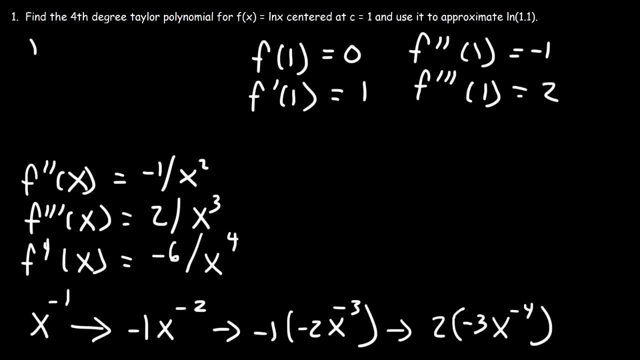 And then finally, for the fourth derivative. This is going to be negative 6 over 1, or simply negative 6.. So now let's write out the fourth degree polynomial. So we said it was f of c or f of 1, which is 0. 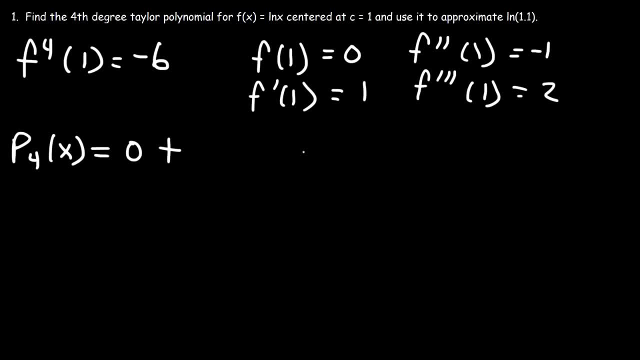 And then plus, it was f prime of c, which is 1, times x minus c, and c is 1, over 1 factorial, which we don't need to write right now. And then it's going to be f, double prime of 1,, which is 1 over 1 factorial. 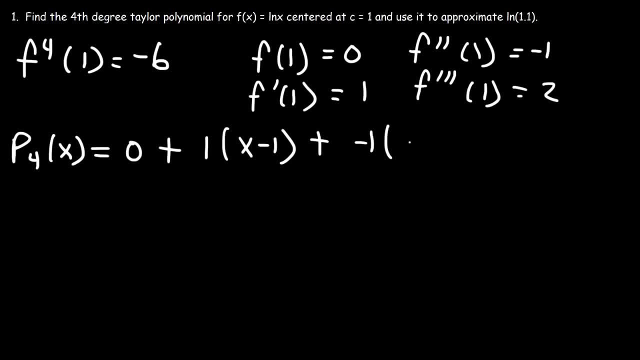 Which is negative, 1, times x minus c squared, or x minus 1 squared over 2 factorial, And then it's going to be f triple prime of 1, which is 2, times x minus c. to the third power: 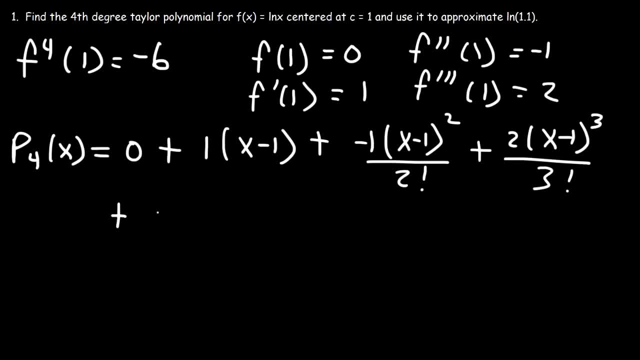 divided by 3 factorial. And then the last term is f, prime of 4, which is negative 6, times x minus 1 to the fourth power over 4 factorial. So now let's simplify what we have, So we don't need to worry about the 0. 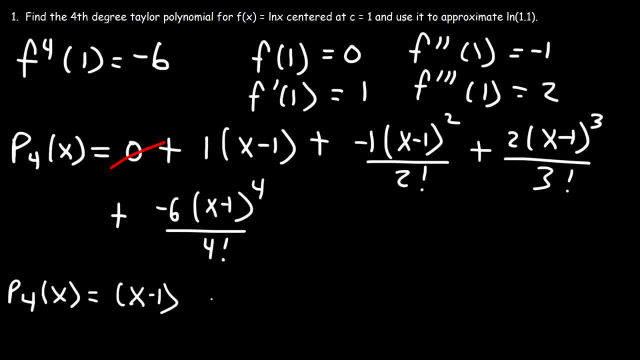 And so the first term we have x minus 1, and then this is just negative 1 over 2.. So we can write that as negative 1 half x minus 1. squared Now, what is 2 divided by 3 factorial? 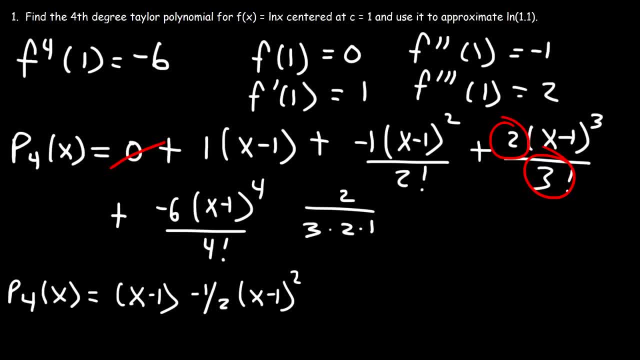 3 factorial is 3 times 2 times 1.. 3 factorial is 3 times 2 times 1.. So we can cancel a 2, and we're going to get 1 over 3.. So this is going to be plus 1 third x, minus 1 to the third power. 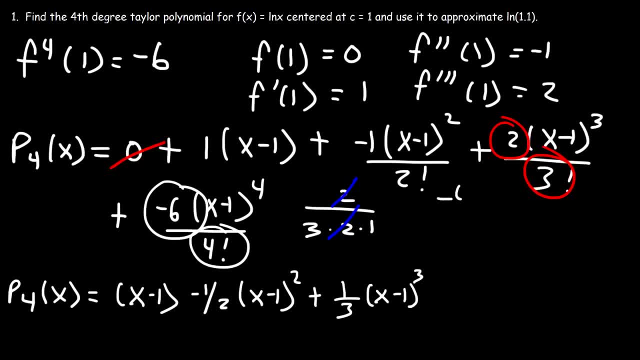 And then we need to simplify negative 6 over 4 factorial. So 4 factorial is 4 times 3 times 2 times 1.. And so 6 cancels with 3 times 2.. And so we're left with negative 1 fourth x minus 1 to the fourth power. 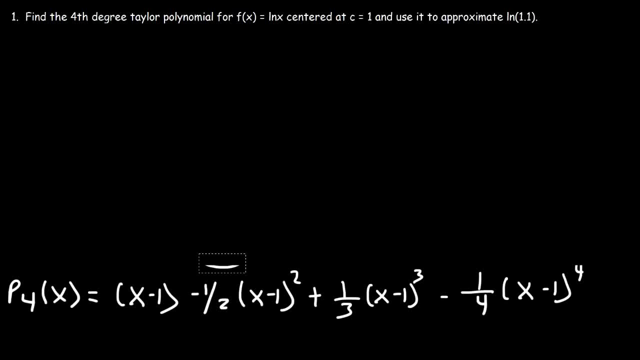 And so this is the fourth degree Taylor Polynomial. So now let's use it to approximate ln 1.1.. So plug in 1.1 into this expression. So 1.1 minus 1 is 0.1.. So this is going to be 0.1 minus 1.1.. 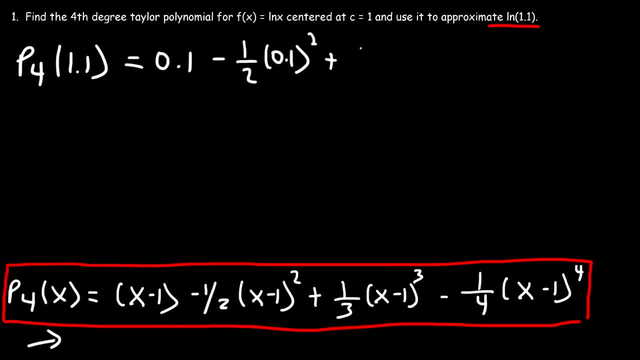 1 half of 0.1 squared plus 1 third of 0.1 cubed, minus 1 fourth of 0.1 raised to the fourth power. So go ahead and type that in. So I got 0.0953083333.. 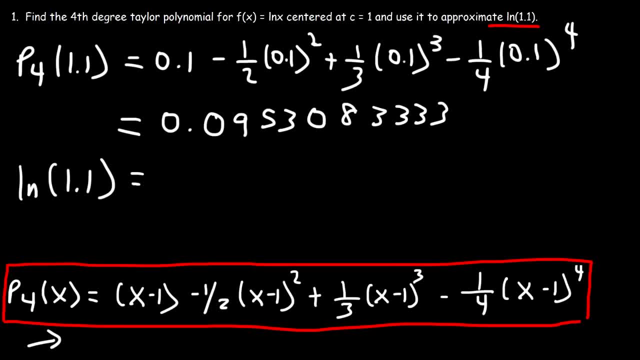 Now let's get the exact answer. So the natural log of 1.1 is 0.0953101798.. So you can see that both answers are very close. So we can round this and say it's about 0.0953083333. 0.09530101798. 0.09530101798. 0.09530101798.. 0.09530101798.. 0.09530101798.. 0.09530101798.. 0.09530101798.. 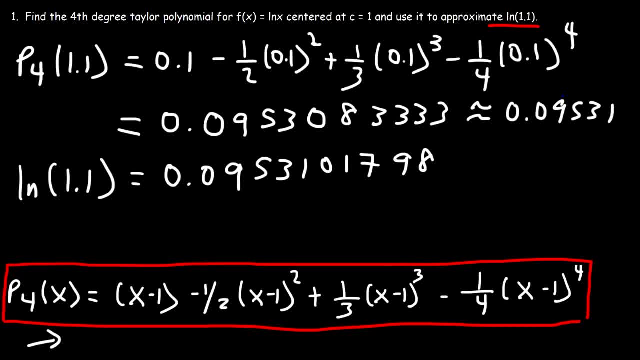 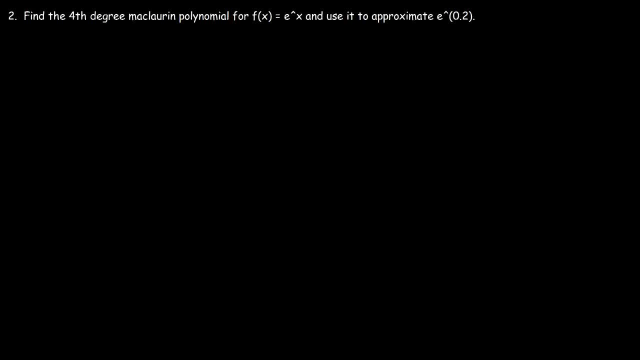 And that would be a good estimation of the natural log of 1.1.. Now let's work on this one. Find the fourth degree Maclaurin polynomial, for f of x is equal to e to the x, and use it to approximate e to the 0.2.. 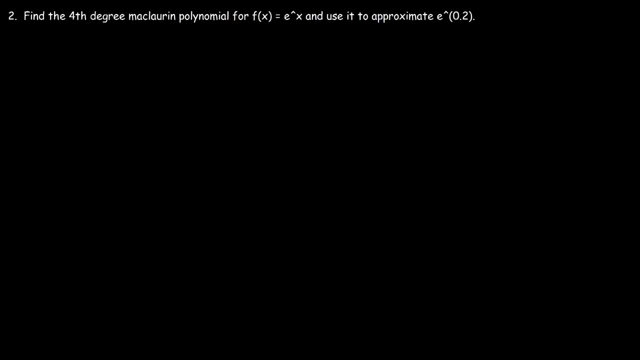 So the Maclaurin polynomial is basically the Taylor polynomial, centered at 0. That's the only difference. So you could use the same formula, but c is equal to 0.. So let's write the general formula first for the f degree polynomial. 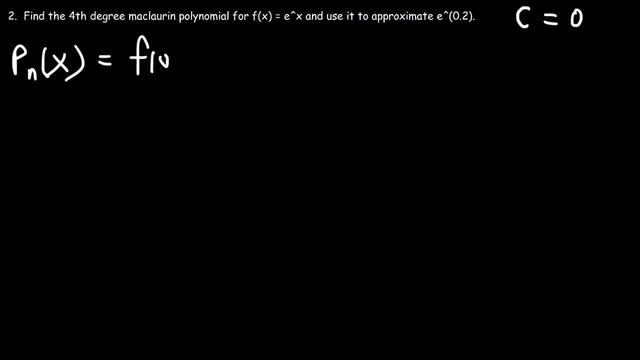 So instead of f of c, it now becomes f of 0. And instead of f prime of c times x minus c, it's now f prime of 0 times x minus 0, which is simply x. So this is going to be x to the first power. 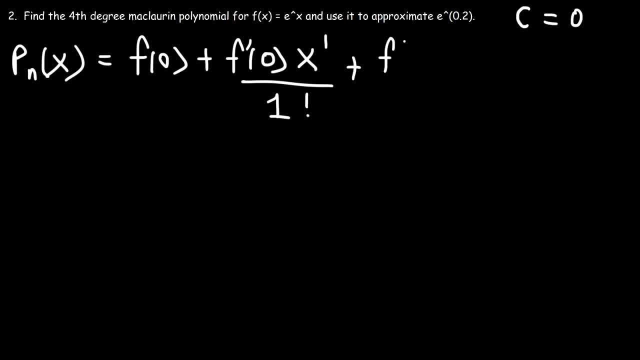 Over 1.1.. Okay, And then it's going to be the second derivative f double prime of 0 times x, squared over 2 factorial, And this trend will continue until you get to the f degree where you want to stop times. 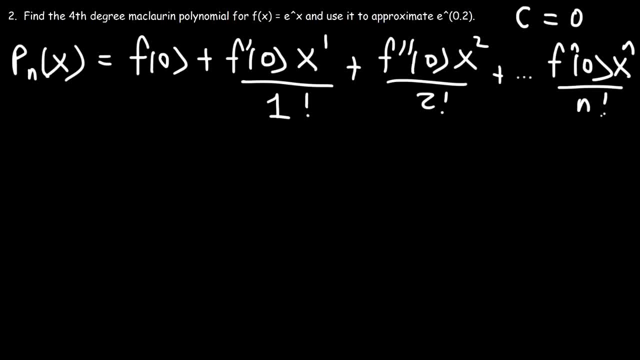 x to the n over n factorial. Now f of x is e to the x, And f prime of x is also e to the x, And this will just continue. So f of 0, which is e to the 0,, that's 1.. 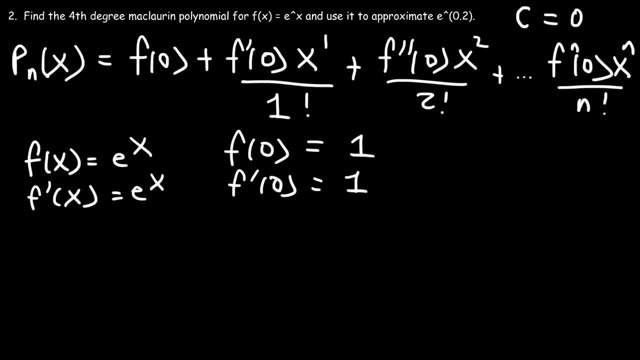 And so f prime of 0, that's going to be the same thing. So f double prime of 0 is also 1.. F- triple prime of 0, that's 1 as well. So we're looking for the fourth degree polynomial. 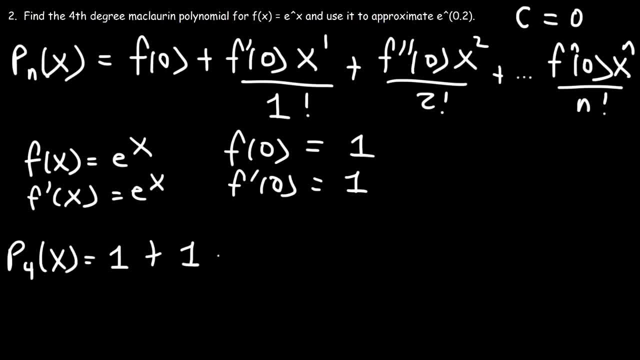 And so f of 0 is 1.. And then f prime of 0 is 1 times x over 1 factorial, And then f double prime of 0, that's going to stay 1.. And then that's going to be x squared over 2 factorial. 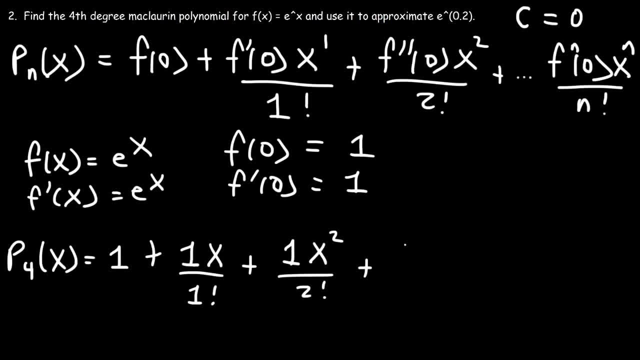 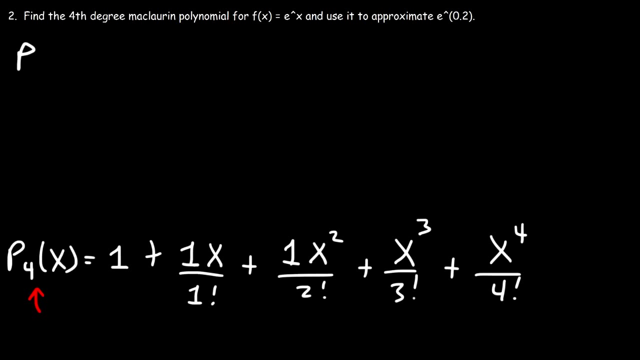 And then it's going to be f triple prime of 0, that's going to be 1 as well. Then it's going to be x cubed over 3 factorial, And then x to the fourth over 4 factorial, And we're going to stop at 4.. 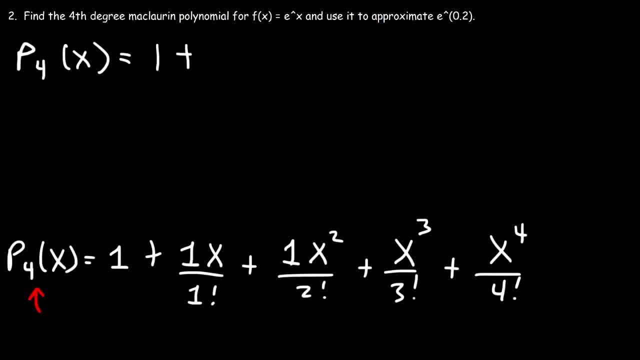 So I'm going to rewrite this expression. So I'm going to rewrite this expression. So this is 1 plus x plus x squared over 2 factorial, plus x cubed over 3 factorial, plus x to the fourth over 4 factorial. So now let's use our fourth degree Maclaurin polynomial to approximate this expression. 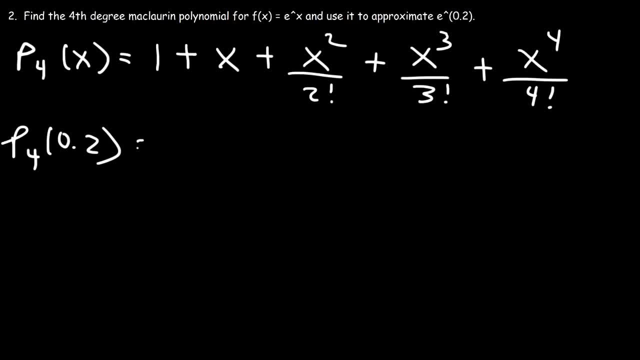 So let's plug in 0.2.. So this is going to be 1 plus 0.2, plus 0.2 squared over 3 factorial Over 2 factorial, plus 0.2 cubed over 3 factorial, and then plus 0.2 to the fourth power over. 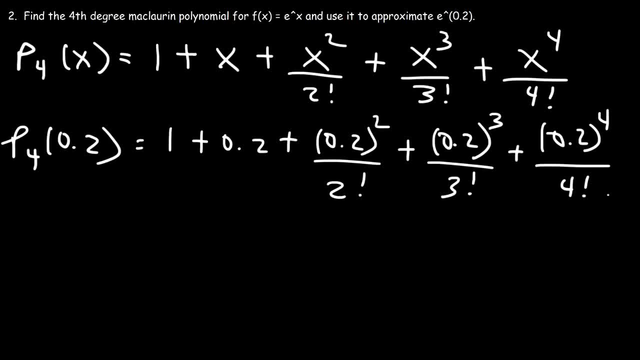 4 factorial. So you should get 1.2214.. 1.2214.. 1.2214.. So that's our estimation. And now let's compare it to the exact answer. So e raised to the 0.2, if you type that in, you should get 1.221402758. 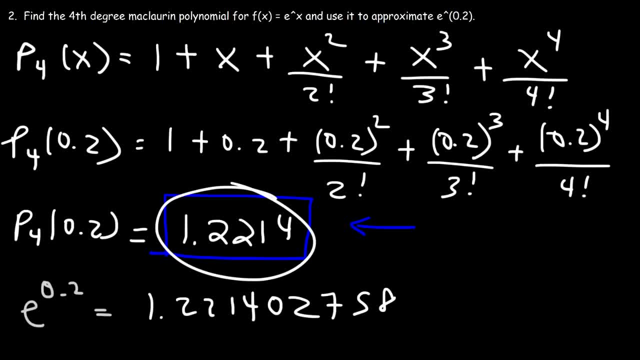 So this is a good estimation of the real answer, And so you could use the Taylor polynomial and the Maclaurin polynomial. And so you could use the Taylor polynomial and the Maclaurin polynomial and the Maclaurin polynomial and the Maclaurin polynomial. 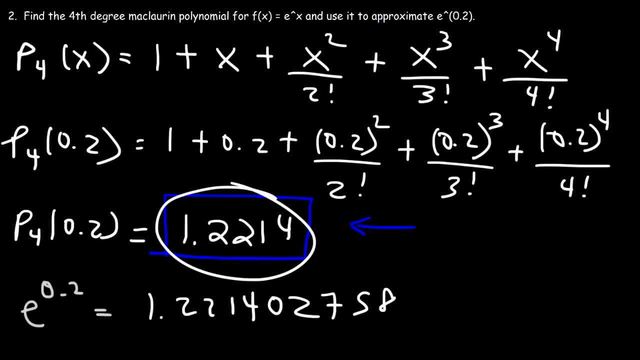 To represent real functions and you can approximate function values when it's close to some central value. In this case, 0.2 is close to 0. This particular function is centered at 0. Now, if you want to increase the accuracy of your approximation, increase the value of n. 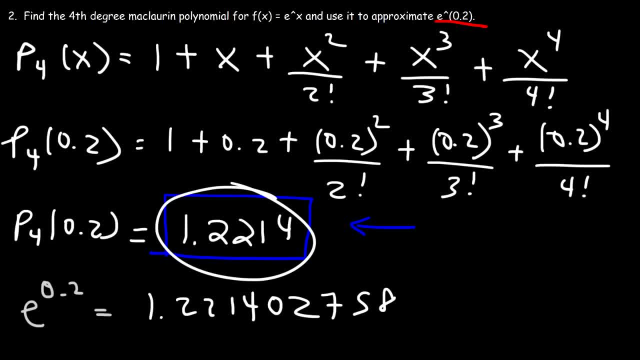 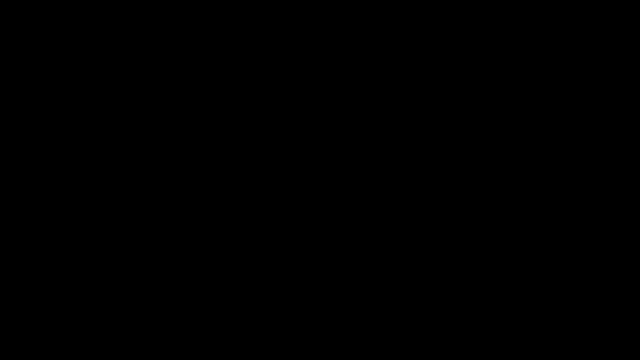 So, for instance, the fifth degree polynomial is going to give you a better approximation than the fourth degree polynomial. It's going to give you a better approximation than the third degree polynomial. So, for instance, there's an penalty for your first deduction, let's say at 15 different. 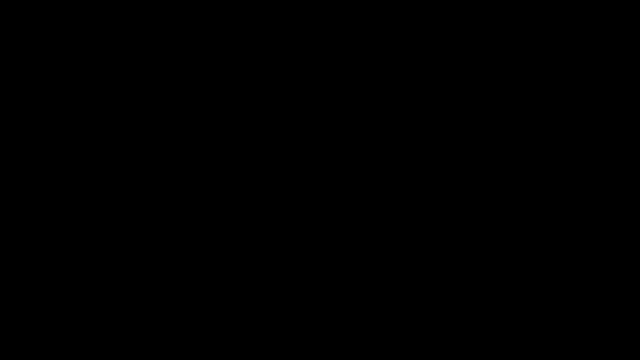 ariest value. Now, that's not the solution, and let's go do a nightmare. 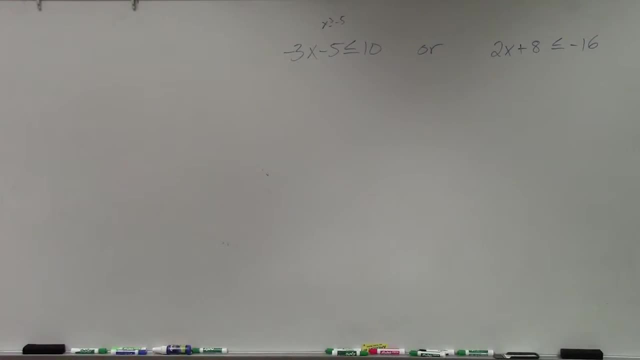 So now and in your problems, ladies and gentlemen, you're going to have three different types of inequalities: compound inequalities. You're going to have ones that are already joined, like the one I did before. You're going to have ones that are going to look.